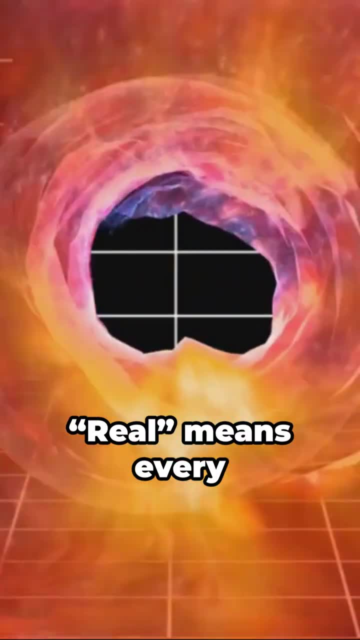 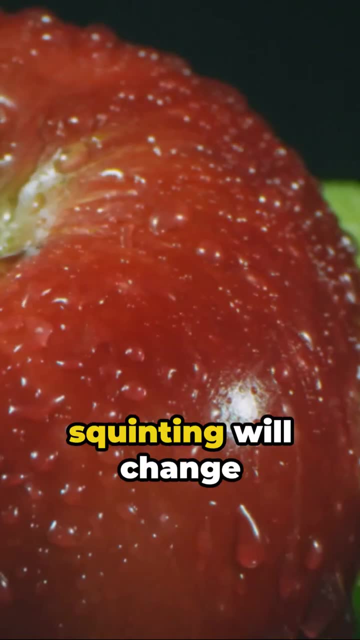 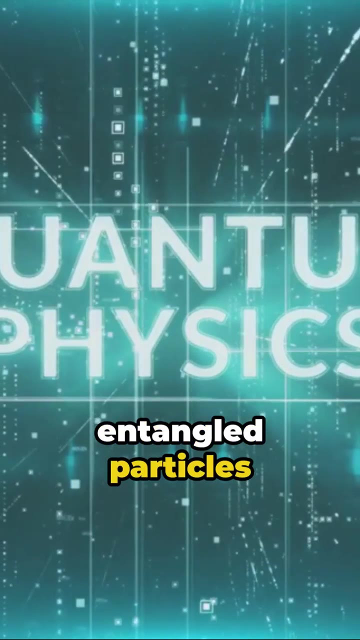 surroundings, not by happenings on the other side of the universe. Real means: every object has definite properties, regardless of how it is observed. No amount of squinting will change an apple from red to green, Except careful. repeated experimentation with entangled particles has conclusively shown such seemingly sensible restrictions. 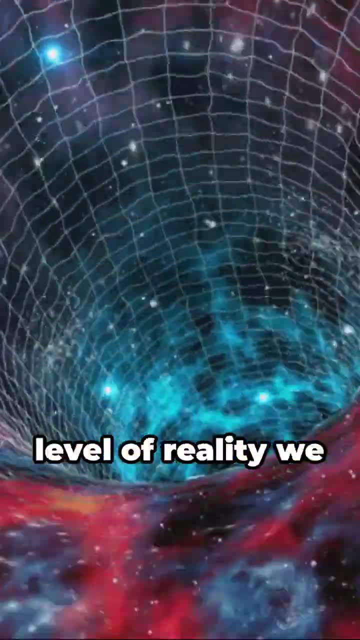 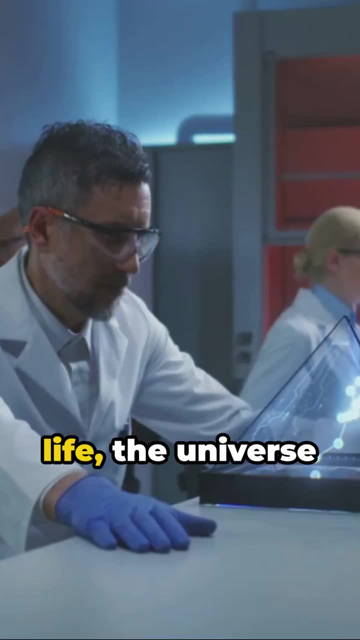 do not always apply to the quantum realm, the most fundamental level of reality we can measure. If you're uncertain as to what exactly the demise of local realism means for life, the universe and well everything, don't worry, You're not alone. Physicists are befuddled.